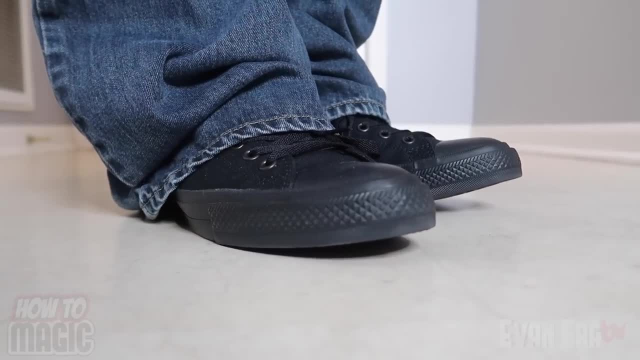 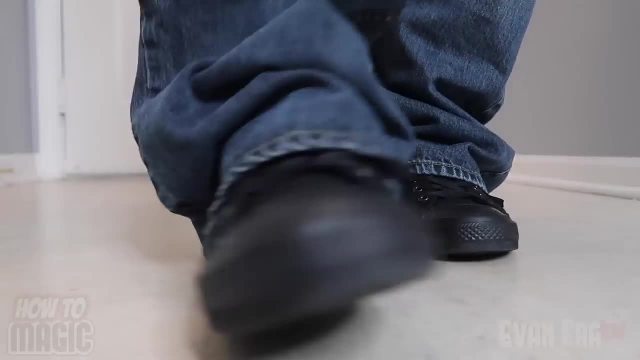 time. It's a classic magic trick. It's really amazing if you practice it in the mirror and make sure you get it right first, so that when you show people it looks like you're really floating. And that is the secret behind the magic Balducci levitation. Here's another. 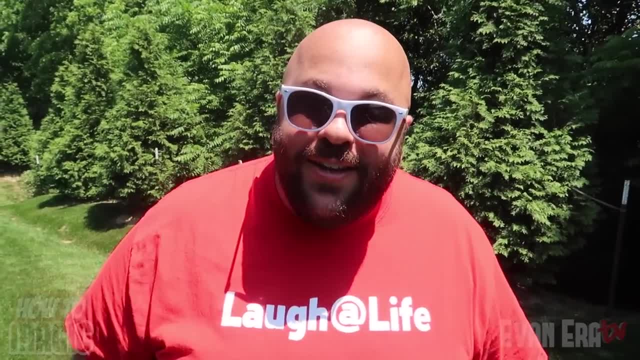 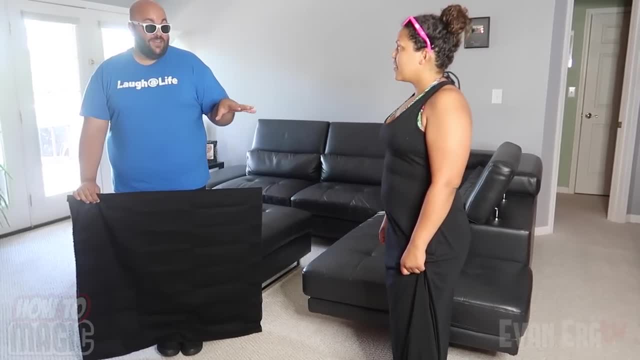 classic way to make yourself float that you can do at home. Take a look. Okay, Veronica, I have a really cool trick to show you. Have you ever seen someone float before? No Levitation. No, You know what levitation is? No Watch, See my feet poking out of the bottom of the 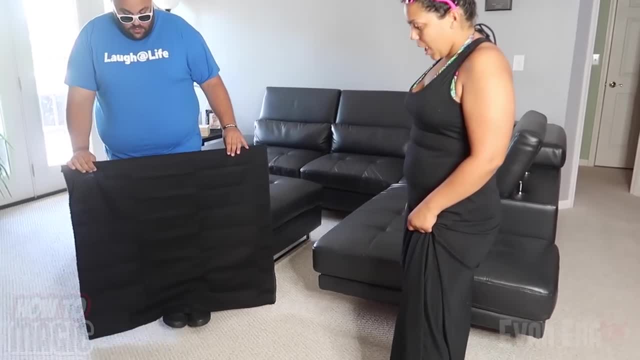 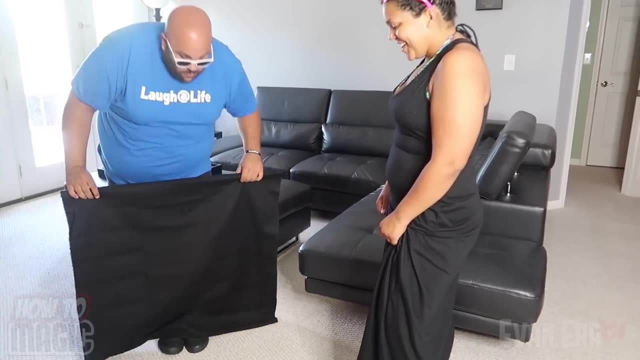 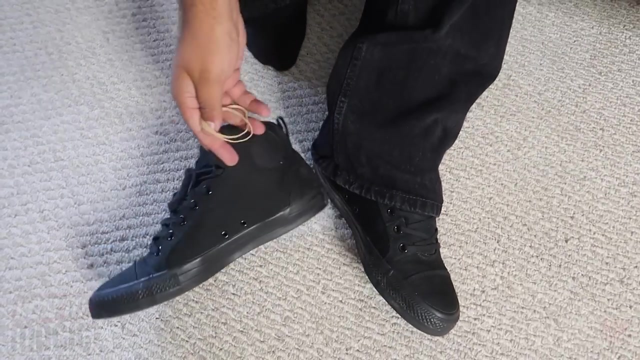 chair right there. No, Check this out. Oh my God, What? Here's the secret behind this amazing magic trick. The setup for this is really simple. You're going to kick off one shoe and you're going to take a couple rubber bands and rubber band your shoes together. 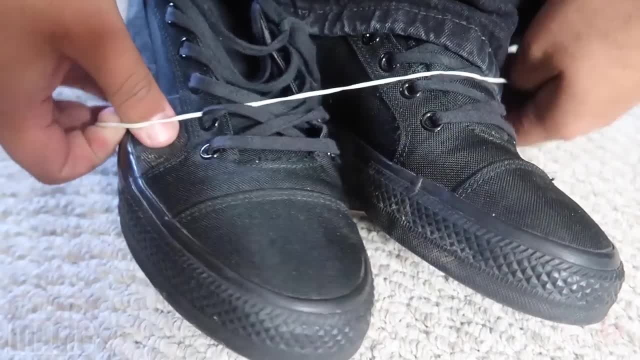 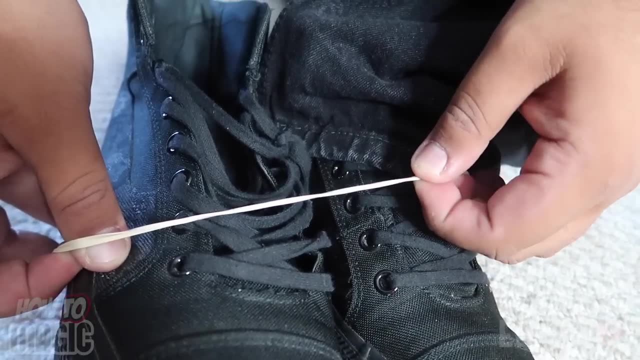 You're going to do this before the trick starts out of your spectator's view. obviously, I'm doing this with a light colored band on top of black shoes for demonstration purposes, But when you do it in real life, you're going to want to get white shoes or a matching color. 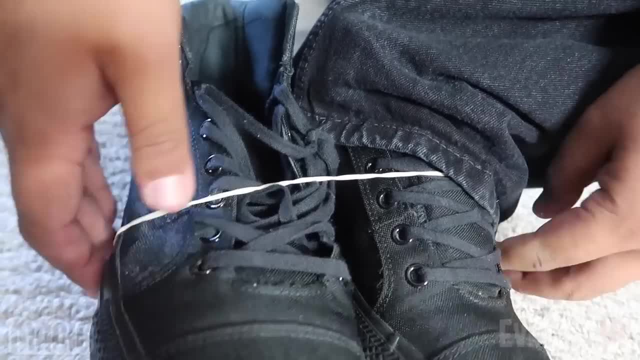 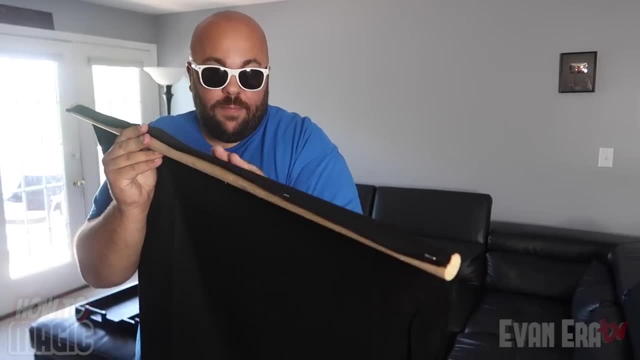 rubber band to match the color of shoes that you have on, so they blend in. Got the rubber bands wrapped around There, you're good to go, All right. so you need a black curtain. That's the second thing you need. It's a dowel rod and then we staple, gunned, a piece of black. 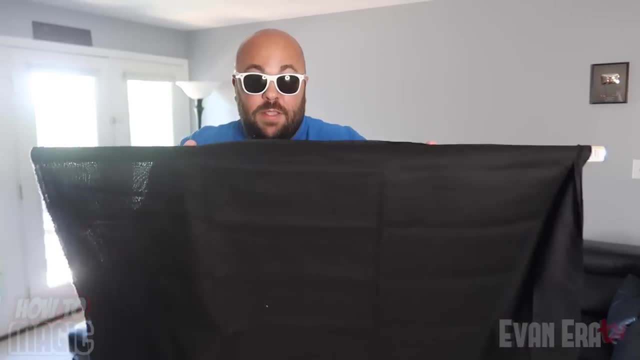 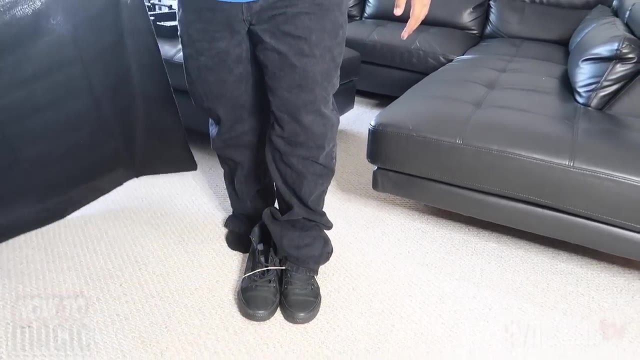 fabric to it. Get a piece of black fabric for a couple dollars. You're just going to staple, gun that to your dowel rod and you've got this nice magic curtain now. So what this black curtain is going to do is provide cover, but they don't see this set up with your legs. 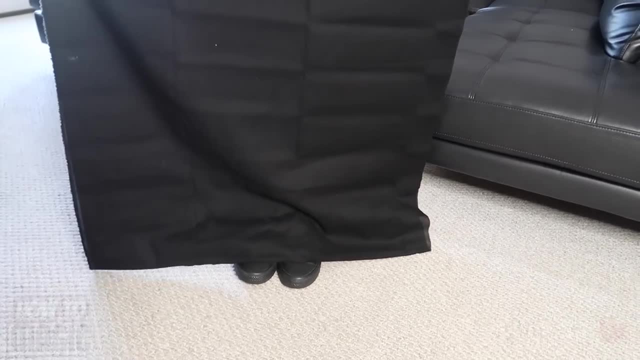 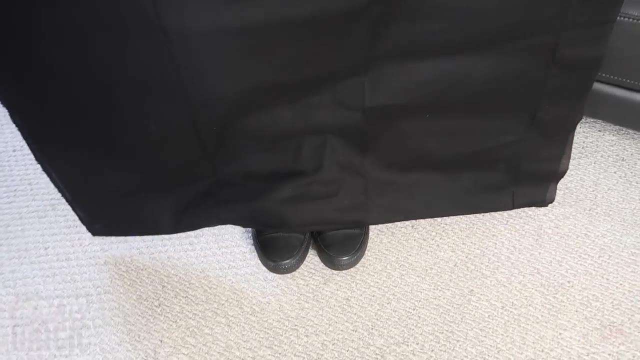 Your feet pointing out of the bottom of the curtain. So to them they think you're just standing normal, because from the waist up you look completely normal and the tips of your shoes look completely normal too. What they don't see is you standing on the other. 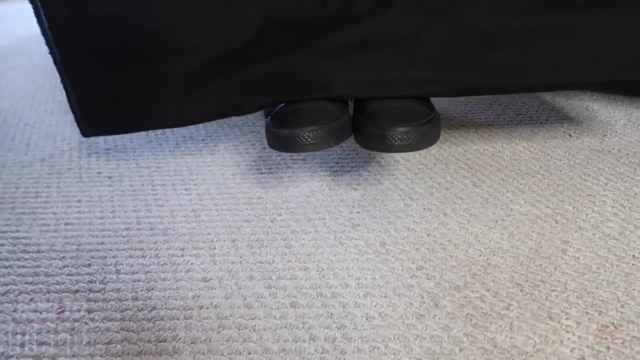 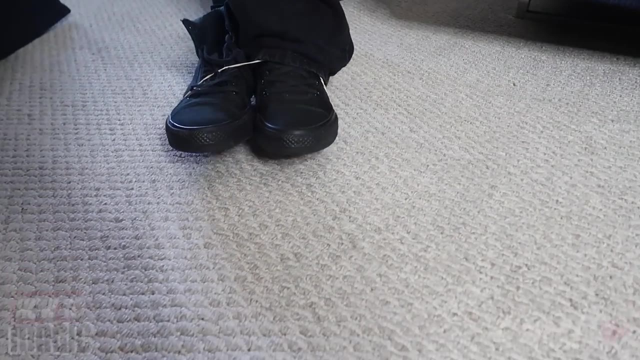 leg to lift up your shoes, to make it look like you're floating in midair, So from an exposed view, slowly lifting up my leg and you look like they're floating, and then slowly lowering them back down. If you want to, you can slip your other foot back into the other. 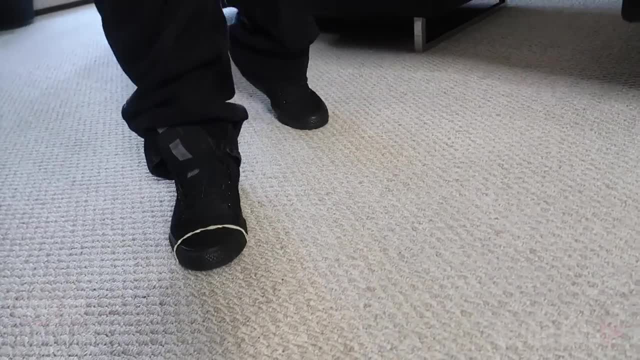 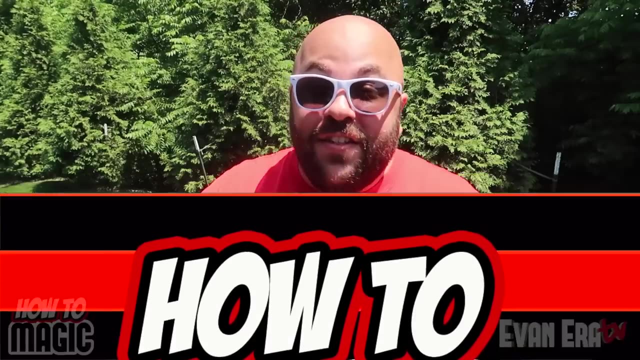 shoe, slip the band off and then step away clean. Oh my gosh, And that is the secret behind the magic floating curtain. Okay, this one is a fun optical illusion that makes it look like you're floating in midair. Check it out. 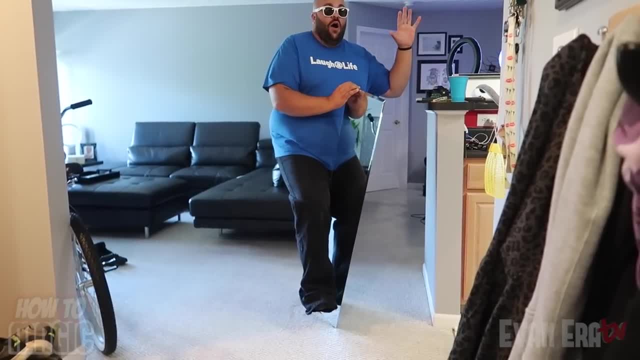 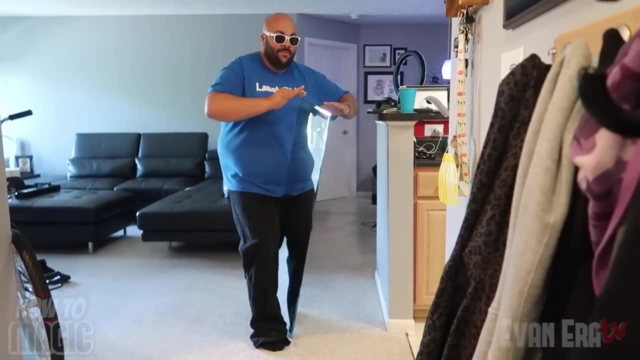 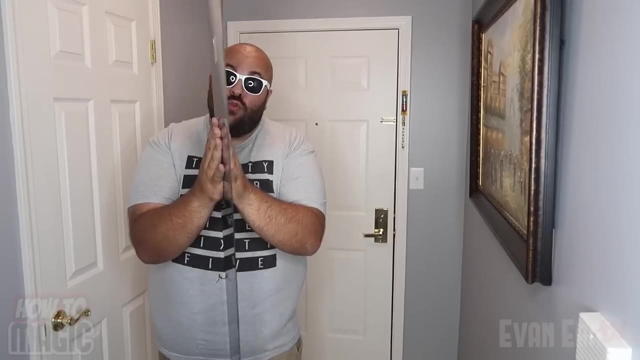 Okay, here's the secret behind this crazy illusion. Okay, the secret to this one is a mirror. All you need is a full length mirror like this, And this trick is all about how you position it. An optical illusion, It's another type. 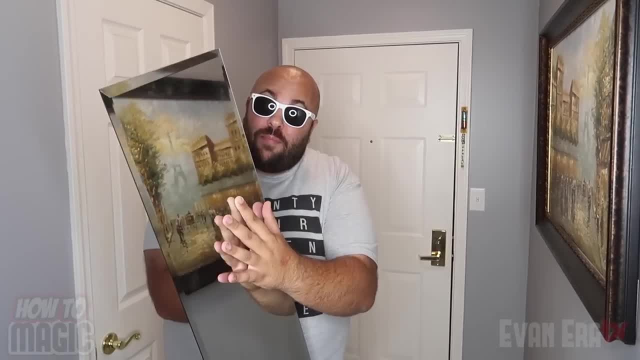 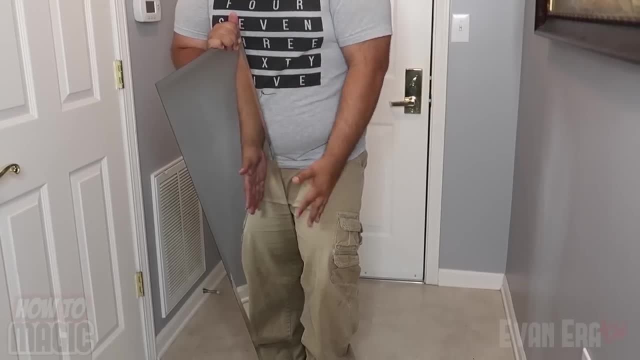 of fun magic trick that would be great to do through a text message. You could take a picture, text your friend and freak them out, making them think that you have magical power. All you're going to do is position the mirror between your legs. You're going. 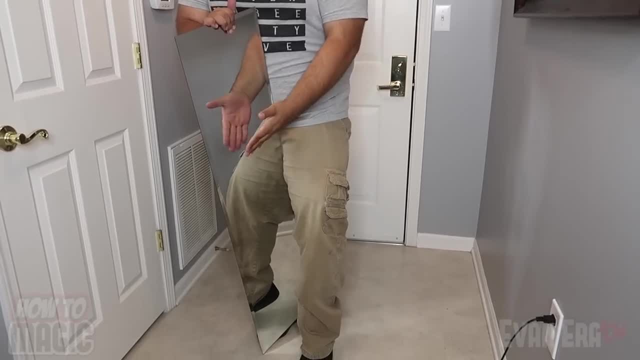 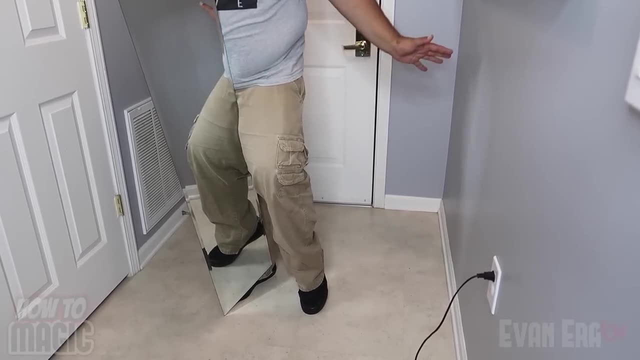 to hide this far leg behind the mirror and put the other leg in front of the mirror, so your leg will reflect in the mirror and create a mirror image of this leg, making it look as if you're just sitting in midair. It's a super cool and fun limitation trick that. 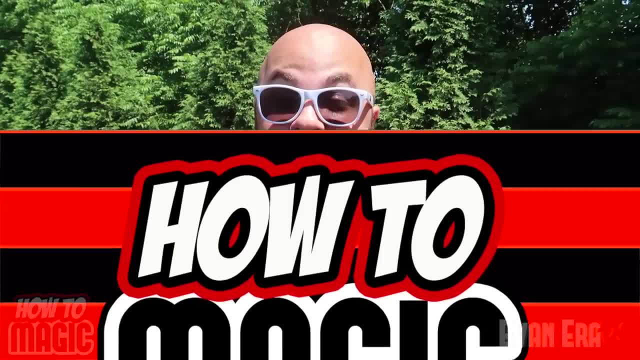 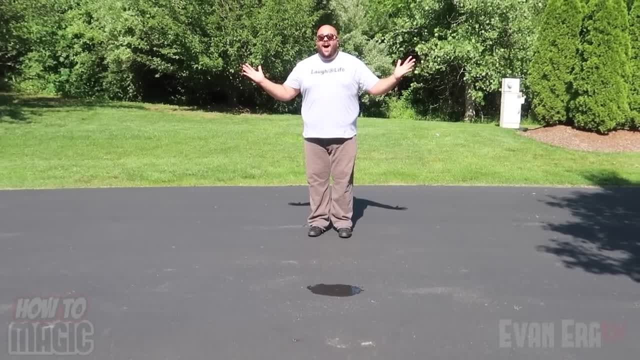 you can try at home And that is how you do the magic floating curtain. Here's a cool way to take a picture of yourself floating and send it to your friends. Take a look: As you can see, the puddle creates the illusion that you're floating. It's all in the perspective. 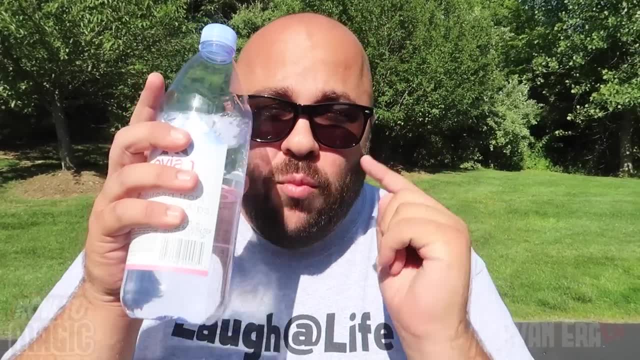 that you're seeing it in the photo. The secret to this one is very simple. All you need is some water. This is totally an optical illusion. It works best as like a text message trick. It's a great photo that you can send somebody. 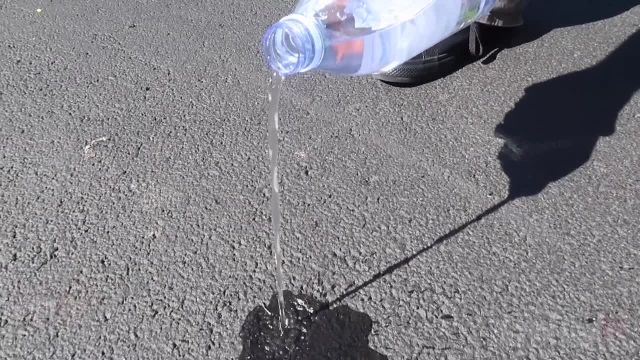 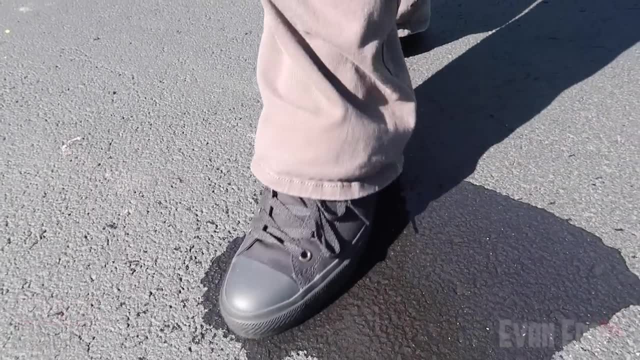 Here's what you're going to do: Take some water. You're going to take some water and pour a little puddle on the ground. You don't want it to be too big, You want it to be about a circle kind of oval shape, Just like that, so it kind of 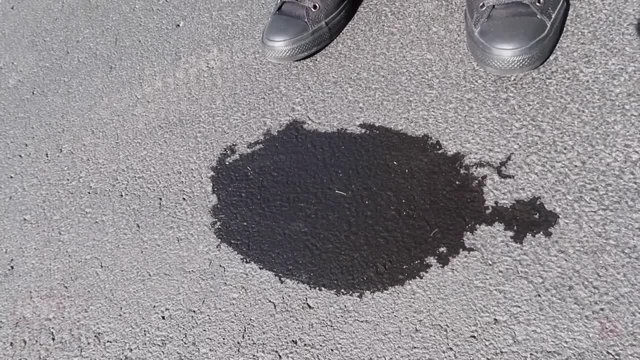 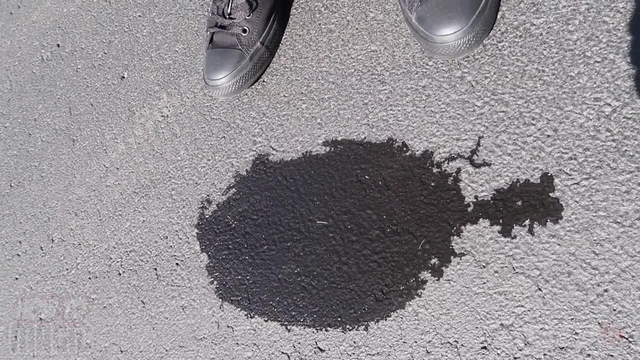 looks like a shadow Puddle on the ground, looks like the shadow beneath your feet, as if you were actually floating. It creates a really convincing illusion that you're just floating in midair. Totally awesome and super easy. And that is how you do the magic puddle of water trick. 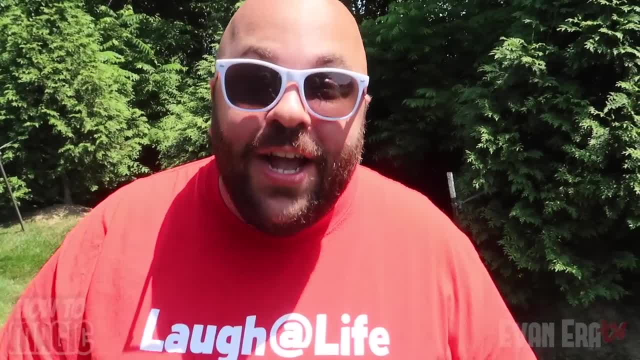 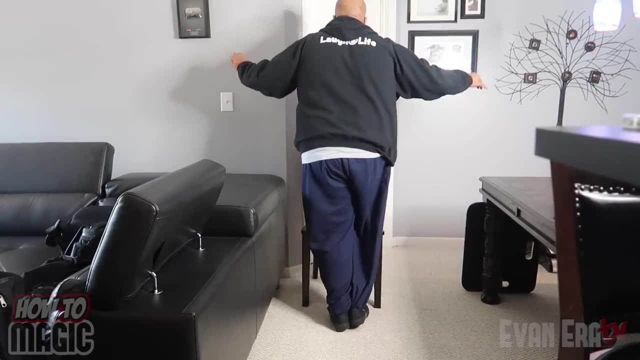 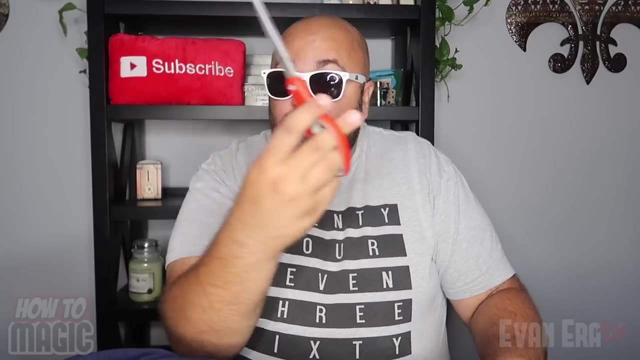 Okay, here's a classic way to make it look like you levitate onto a chair. Check it out. The secret behind this trick is more simple than you might think. Here's an explanation of how it's done. Okay, for this one, you're going to need a pair of pants that you don't mind destroying. 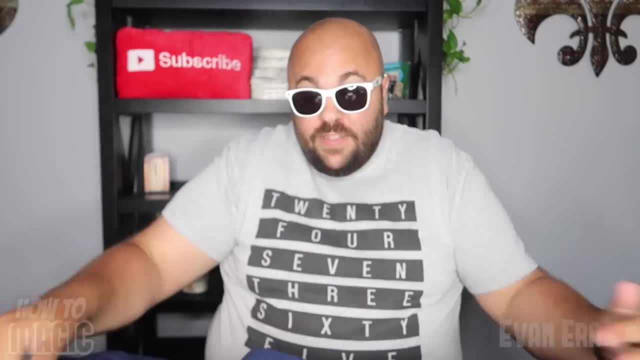 So get an old pair of pants, or go to a thrift shop and get some pants that you don't mind cutting off. So you're going to take some scissors and what you're going to do is cut a slit in the front leg of the pants. 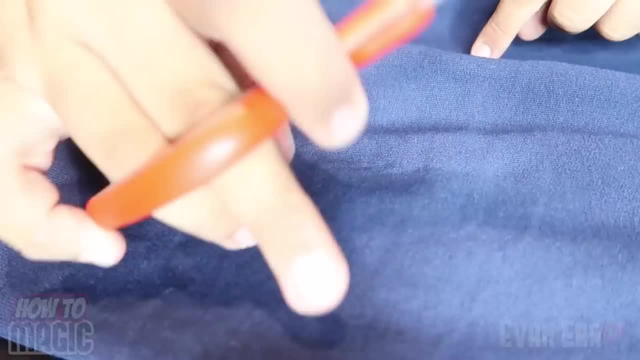 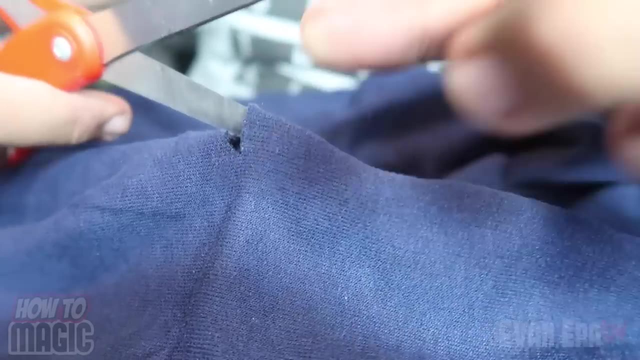 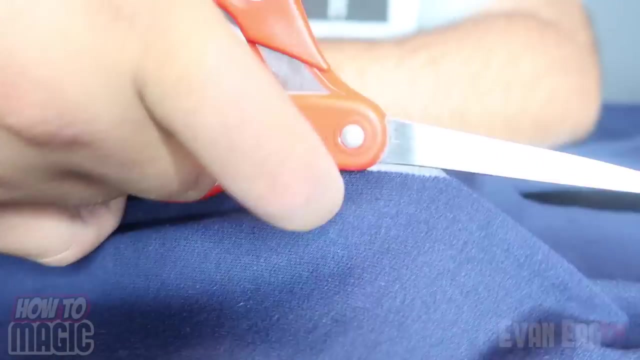 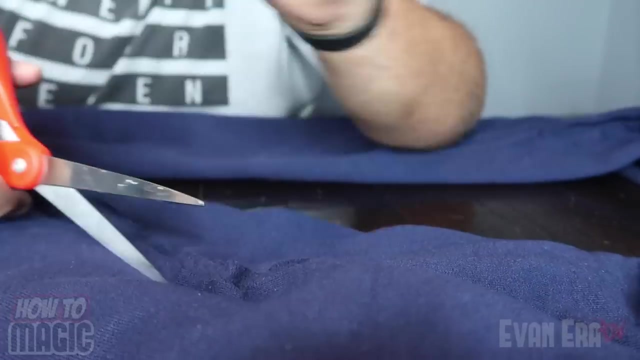 So you're going to find a spot in the fabric right in the middle of the leg. You want to find the middle of the leg right about here And you want to get some pants that are kind of baggy Cut into it. Then you're just going to cut a slit right down the leg. 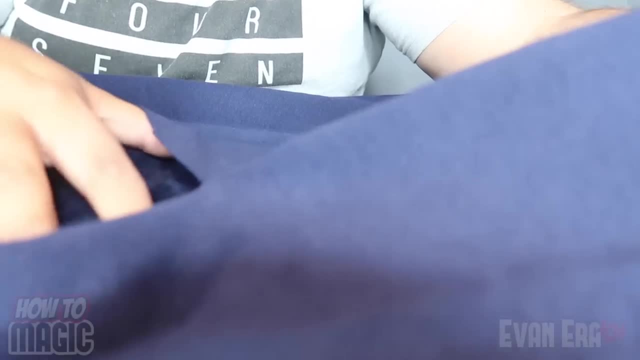 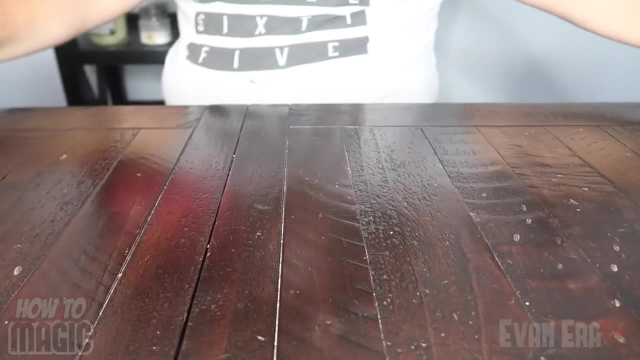 Now, you don't want to cut all the way down the pant leg, You want to stop before you get to the bottom. You just need enough room to slip your leg out. Okay, now that you have your pants cut, the next step is to prepare your shoes. 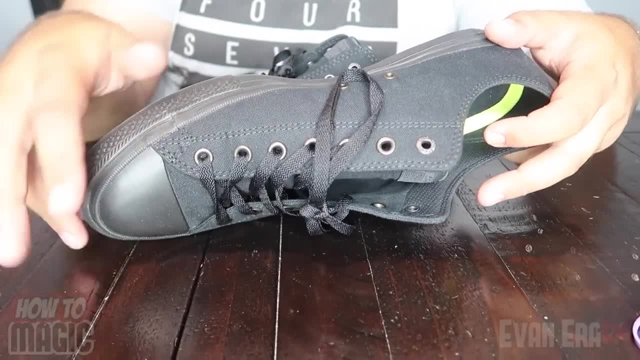 So there's a more advanced set up for this, where you can use a pair of pants. You can use magnets glued on the side of your shoes to stick them together. I'm going to show you a simpler version that you can do at home right now. 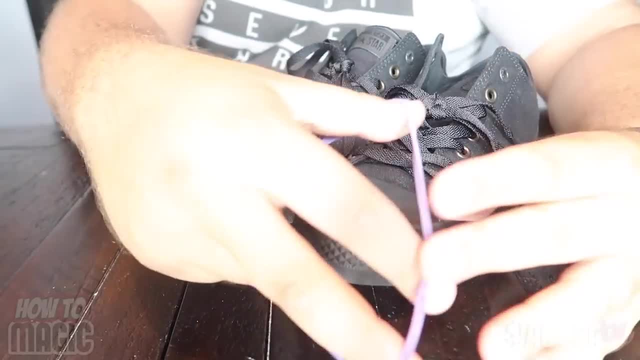 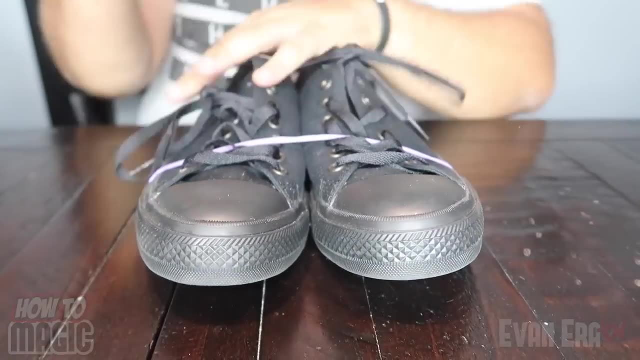 All you do is take a rubber band, just like the other trick, and you're going to rubber band your shoes together. Now you want to use a dark colored rubber band, a black one that would blend in with the shoes when you're actually doing this performance. 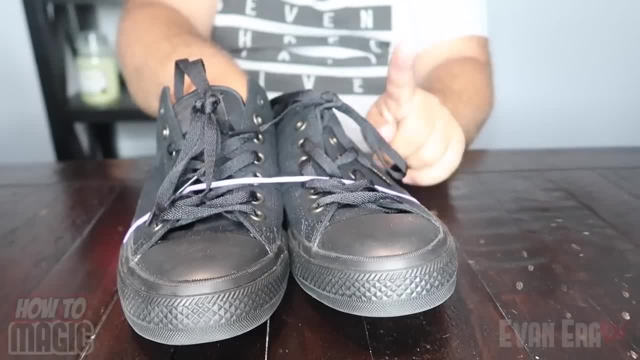 So one foot goes in like this, and it allows both feet to lift up. Here's why that's key. Okay, so you're going to slip your foot into the shoe that has the full pant leg intact. That's this foot right here. 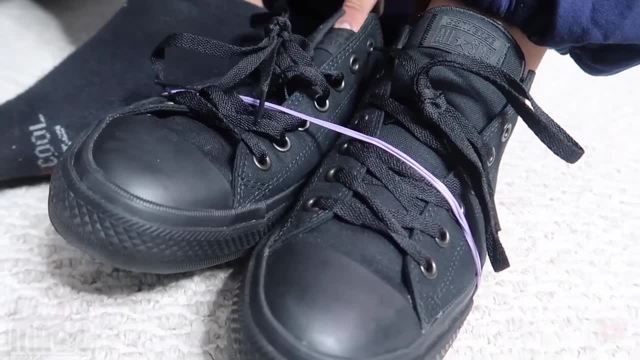 It's not the one with the cut pant leg. The cut pant leg is going to be the empty shoe and your foot's going to stay out of the shoe. So once you have the pants on, this is the full leg of the pants, right here. 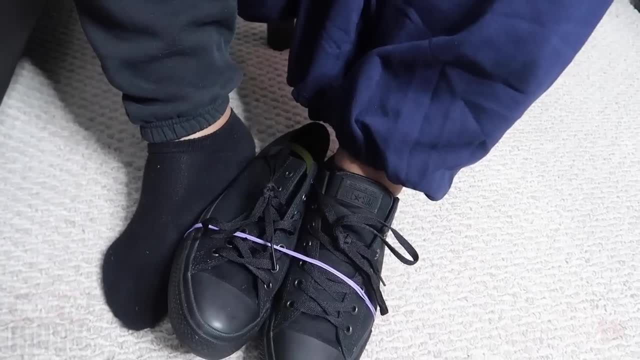 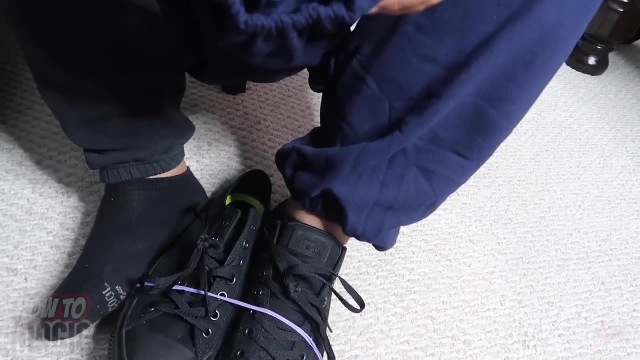 This is the cut leg. You're going to have another pair of dark colored pants on the same color or a similar color to the ones that you're wearing on the exterior with the cut leg. So your foot's going to come out of this and you're going to take this pant leg cuff and 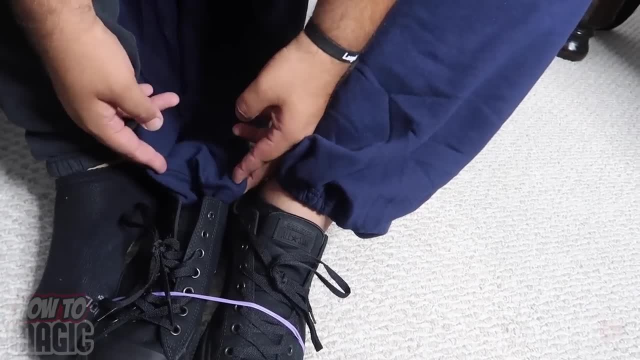 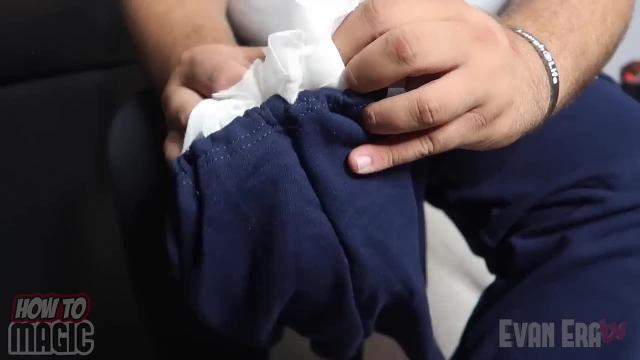 it's going to go down. in the other shoe. You can stuff this full of socks or something like that to give it some form. Okay, So you're going to take some paper towels or some socks and you're going to stuff them into the bottom of your empty pant leg, just like this to give it some form. 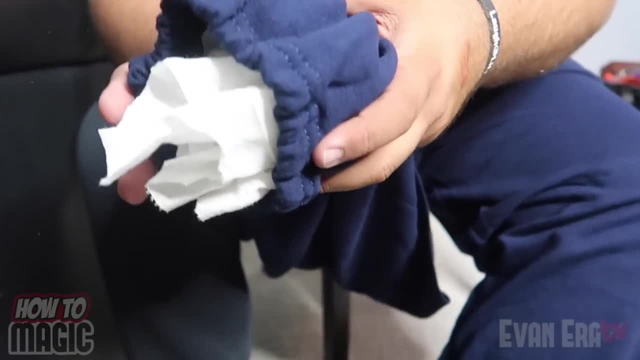 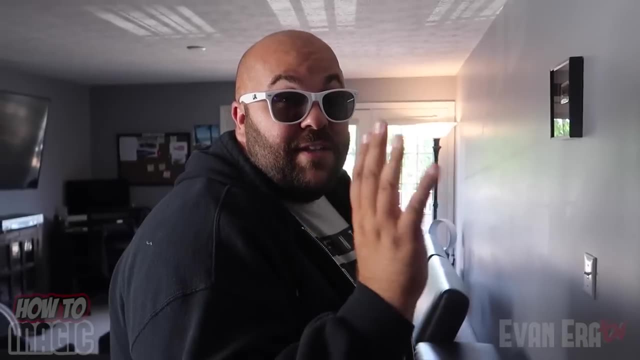 Now we're going to take this and we're going to put it down into the other shoe, Just like that. Now you're in position to do the levitation, So your spectators need to be behind you for this trick. Here's what's happening in the front. 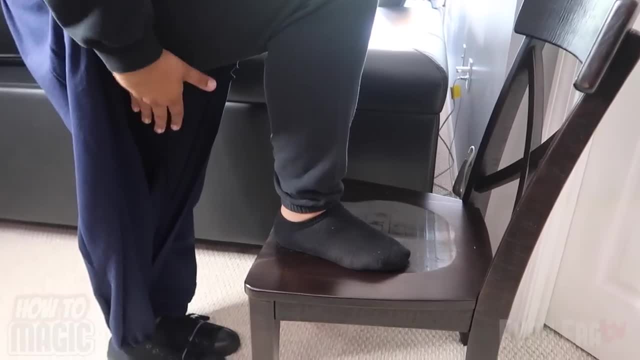 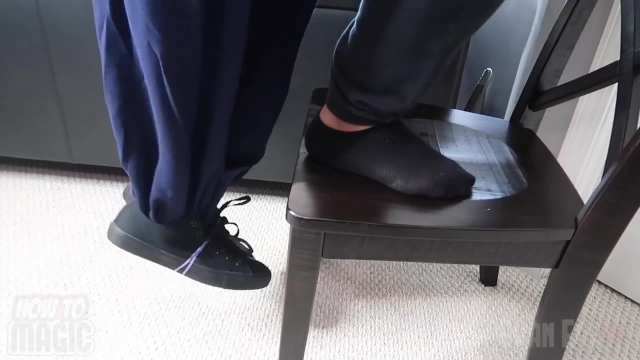 My leg is up out of my pants right here, So this is where the slit comes into play. So I have my leg up on the chair, the two feet banded together. So when I step up onto the chair it looks like I'm floating up onto it from the back. 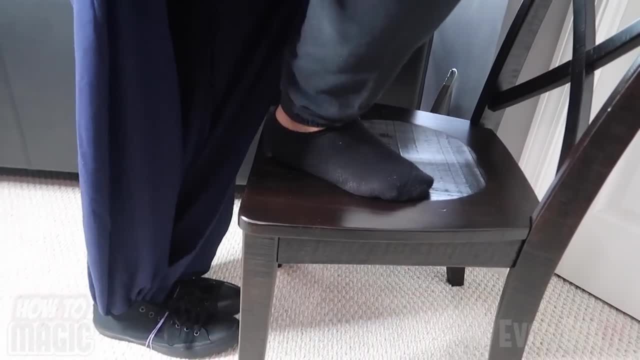 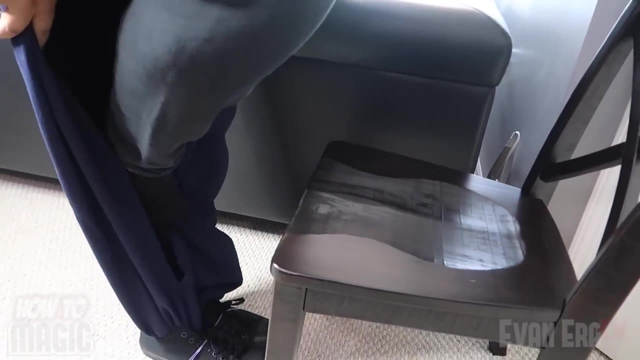 Then when I come back down, it looks like I'm floating back down. It's all done using the power of my leg. I'm just stepping up onto the chair And when you come back down you can slip your leg back into the pants. 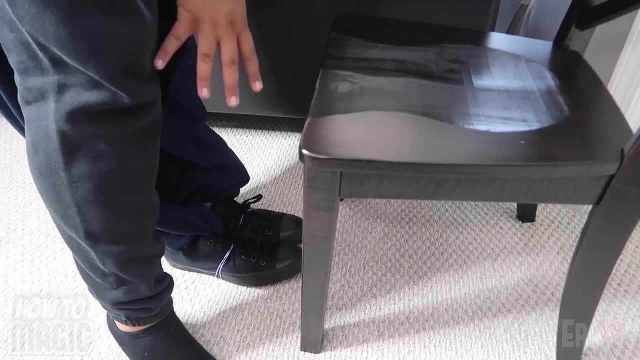 And then the advanced version of this: you can slip your leg into the shoe, separate the magnets and walk away. This is just a fun version that you can do at home and it looks super cool for the people behind you. And that is the secret behind magically floating on the chair. 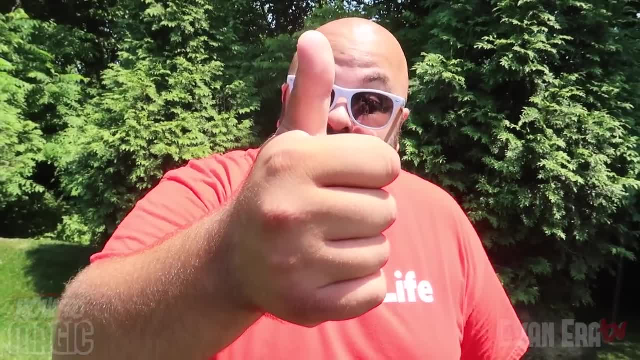 I'm going to show you how to do it. All right, guys, if you liked this video, be sure to give it a thumbs up and head over to howtomagicshopcom and pick up some cool magic tricks that you can do at home. 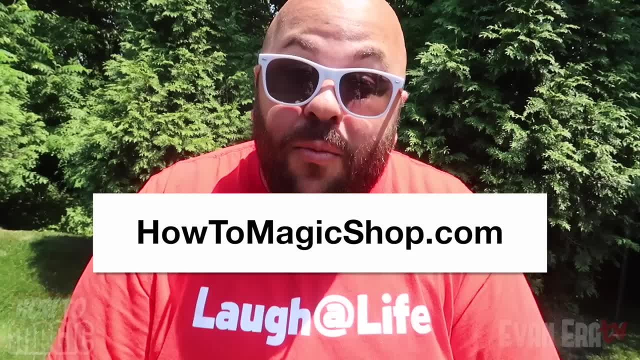 The link for that is in the description of this video: howtomagicshopcom. We have magic tricks in all different varieties. We ship them all over the world. We have international shipping available now, and we also have a lot of cool Laugh at Life. 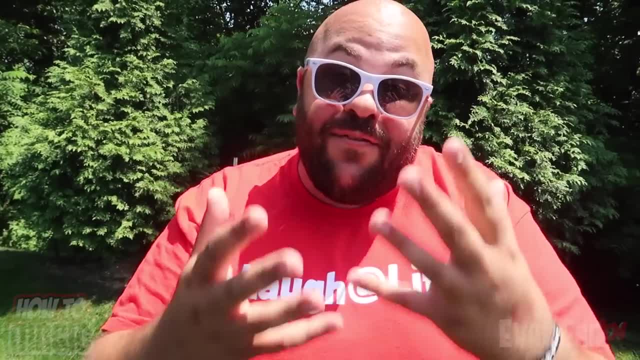 gear for sale. If you want to support the channel and support these videos, help us keep creating fun, magic videos like this one. Pick up some Laugh at Life shades, a bracelet. we have a lot of cool products and we ship them all around the world. 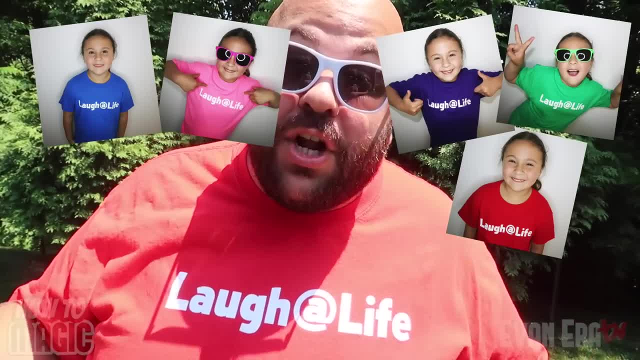 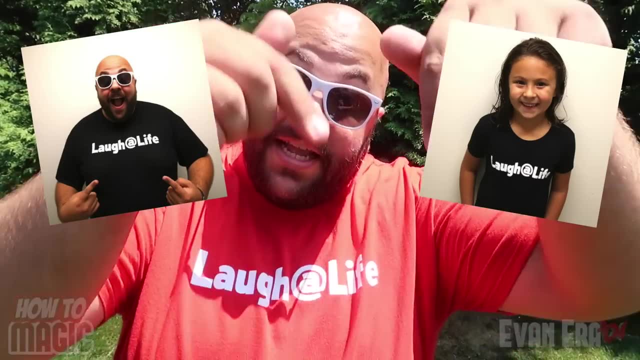 In honor of the launch of our summer collection of all the Laugh at Life tees and these fun summer colors, we are doing the classic black and white Laugh at Life design tee at 50% off for the next 24 hours. If you want to get one, go to the link in the description and pick one up today. while 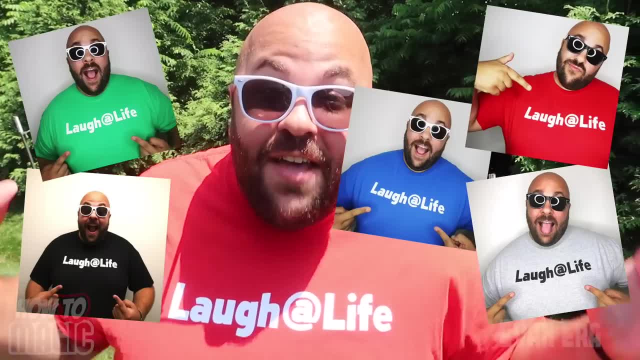 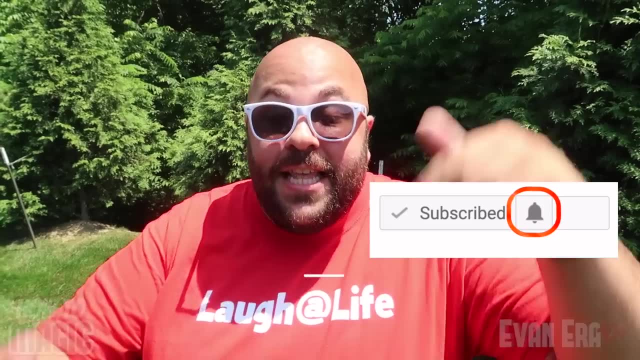 supplies last. All right, guys, it is giveaway time. I'm giving away five Laugh at Life t-shirts to five lucky comments in the comment section below. All you have to do to win is give the video a thumbs up. be subscribed to this channel.